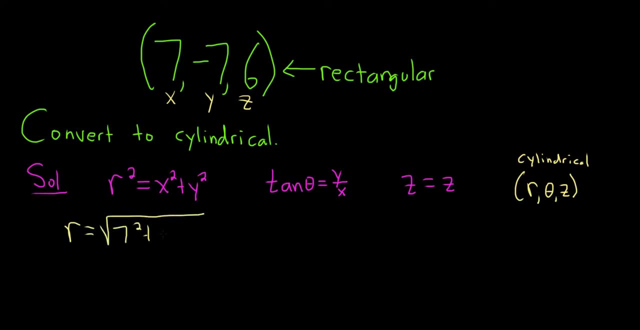 of 7 squared plus negative 7 squared, That's going to be 49 plus 49. And you can add these up. but let's be clever. Watch this: 49 plus 49 is 2 times 49. And why did I do that? 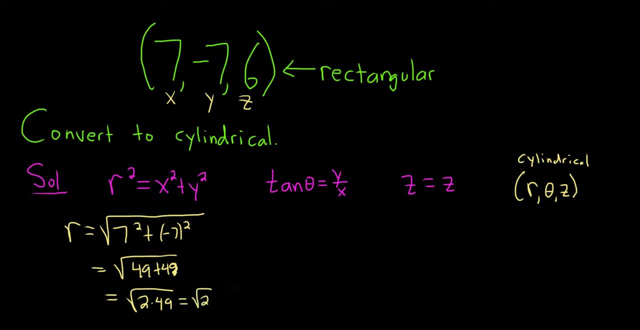 Because now I can do this. This is the square root of 2, the square root of 49.. Just a really, really clever move so that I don't have to use the calculator. So this is 7 squared of 2.. 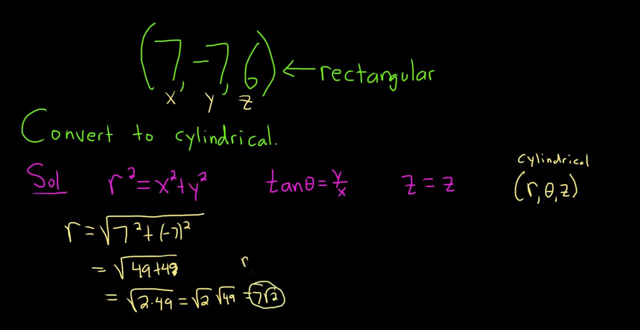 So that's going to be our R. So R is equal to 7 squared of 2.. Again, 49 plus 49 is just 2 times 49.. You have two of them. It's like if you had X plus X. 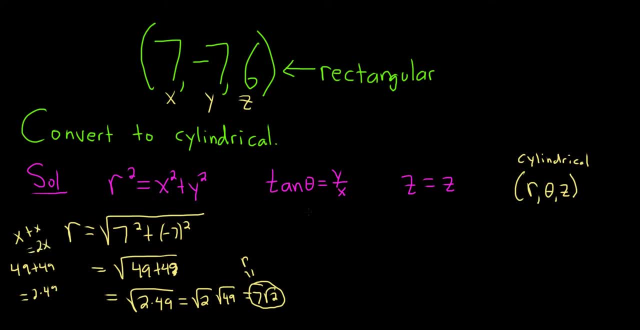 that's 2X. same thing To figure out the tangent of, to figure out theta, we can write down tangent of theta which is Y over X, So it's negative 7 over 7, which is negative 1.. 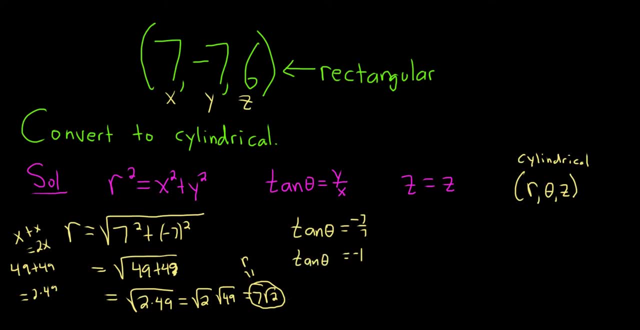 So we have that the tangent of theta is equal to negative 1. Now keep in mind there are infinitely many solutions to this equation, So it's extremely important, when you're finding theta in these problems, to always draw a picture. So I'll do it over here. 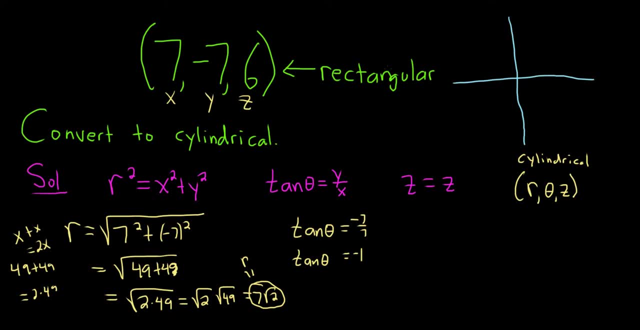 Okay, So our picture will just be a picture of this ordered pair in the XY plane. So we go right 7 and down 7, and that puts us here: Okay, So we have this point here. So you say, okay, what angle is this? 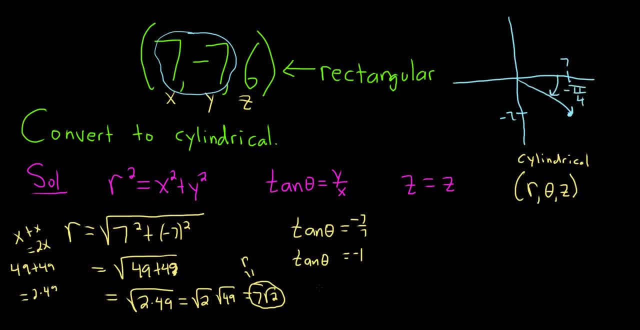 Well, this angle is negative pi over 4. And so that's our theta. So that's the easiest way to figure out the angle, in my view. So let's do this. So always just draw a picture And you could check the tangent of negative pi. 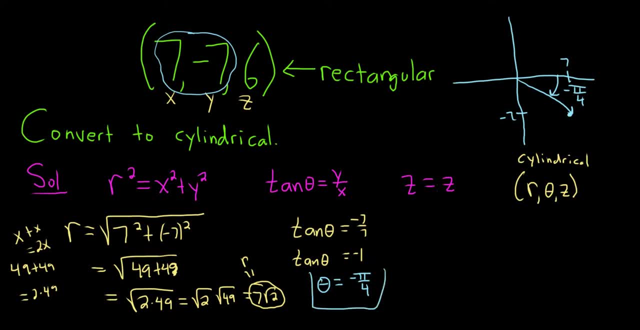 over 4 is actually equal to negative 1.. So super key technique. So always draw a pic, All right. And the last one is Z equals Z Hoorah, That's just 6.. So the final answer, we're done, right.